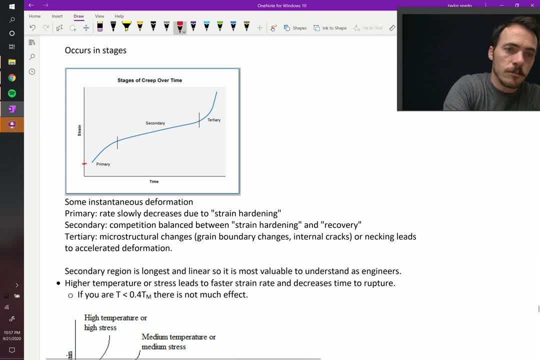 initial strain on you know at time, equals zero. We'll call that strain not. It does initially strain The second: I bend something, it strains, And then if I let this sit for several years, the deformation continues. even under the same load. It grows rapidly at first. 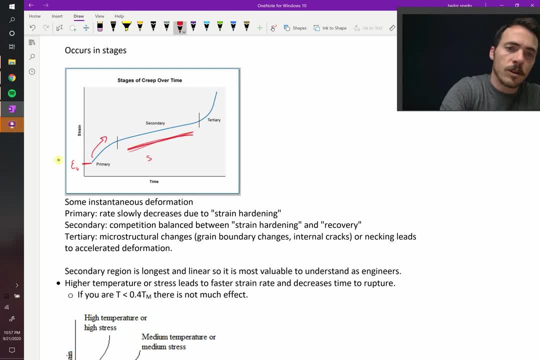 and then it reaches this steady state region. We'll call this steady state. That just means that it's not changing over time. It's a constant rate. The rate is constant there. And then it reaches this tertiary region, which is a rapid onset before it fails in the end, right. 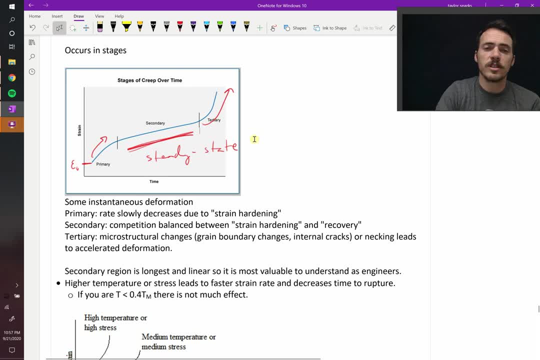 So the thing to know about strain is that it would be useful to understand this steady state region in the center, because then we could predict it right. If we know the rate at which strain's occurring, we could predict how long something will last until it fails, right. So that's primary. 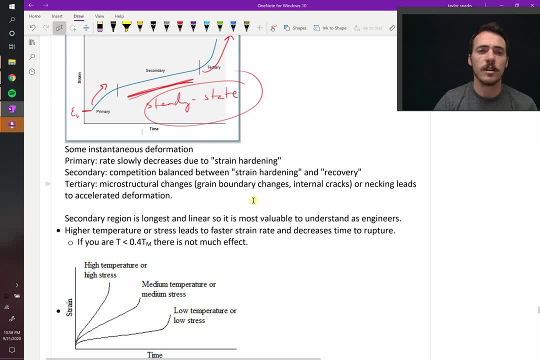 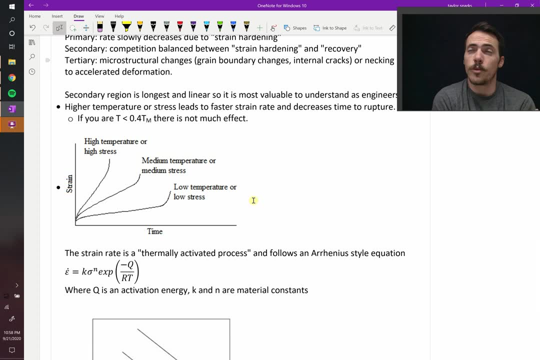 secondary, tertiary and again secondary is sometimes called steady state creep strain. okay. So just like with crack growth, where a larger stress caused a faster crack growth, we see a similar thing here. When you plot strain versus time here you have different slopes. So 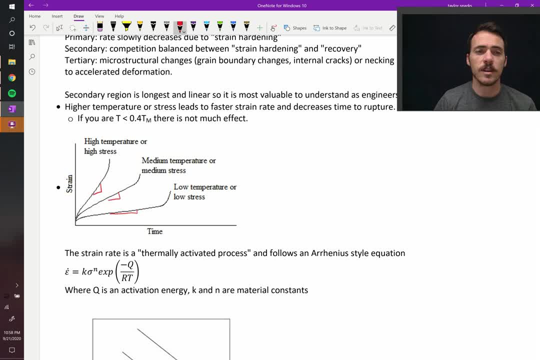 the steady state region is not the same for all these different conditions. At high temperatures or high stress, you get the fastest creep strain rate. At low temperatures and low stress, you get the slowest creep strain rate. okay, Generally this happens at high temperatures. 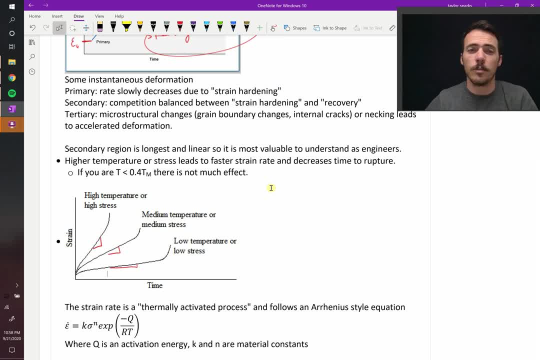 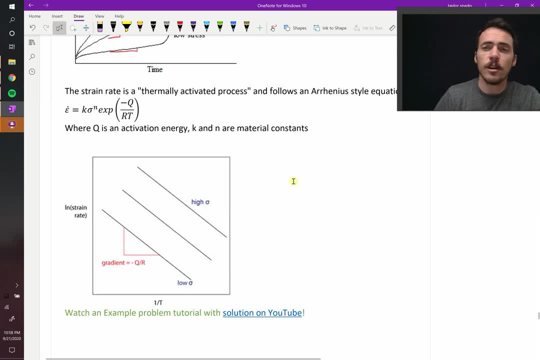 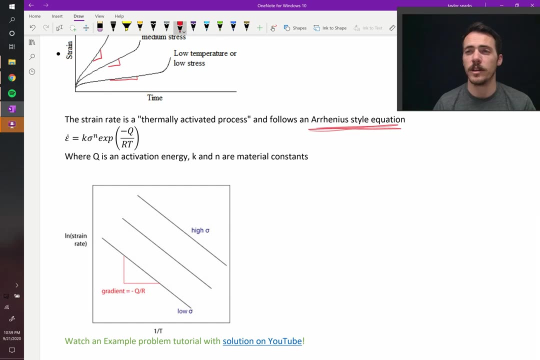 if you're less than maybe like 40% of the melting point, you don't see a large effect here. right, We can model strain rate. It's a thermally activated process. We're going to see so many Arrhenius-style equations, which is some sort of thermally activated process in material science. 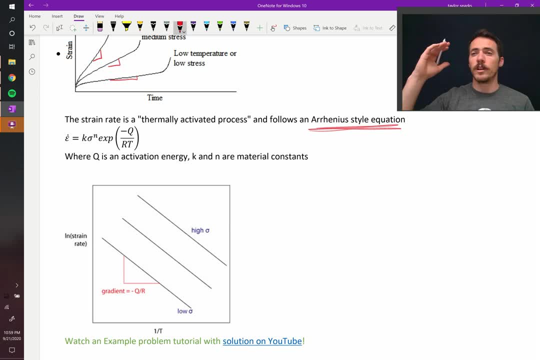 So much of material science is thermally activated, meaning it goes much faster at high temperatures because there's an exponential with an activation energy- q. that's our activation energy, and then you have a rate of strength. So you can model strain rate at high temperatures. but you can also model 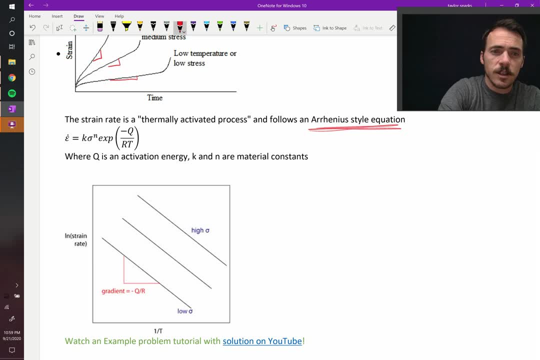 RT, R is the gas constant, T is temperature, And then, in this case, the strain rate, epsilon with a dot on top. that means the rate of strain. so the rate at which it's deforming is equal to k, a constant times sigma, the applied stress. 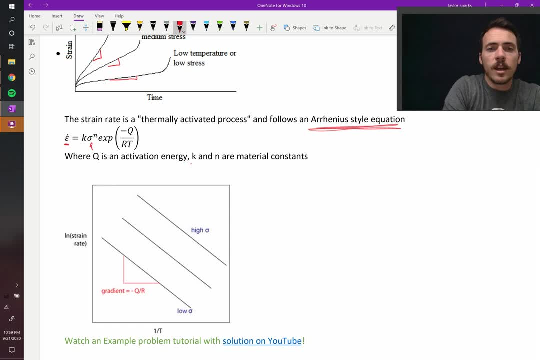 right, that's our stress to the n, So k and n are going to be materials constants, as is the activation energy. Now how do we figure these things out? There's lots of ways to do it. You could take this equation and you could linearize it. 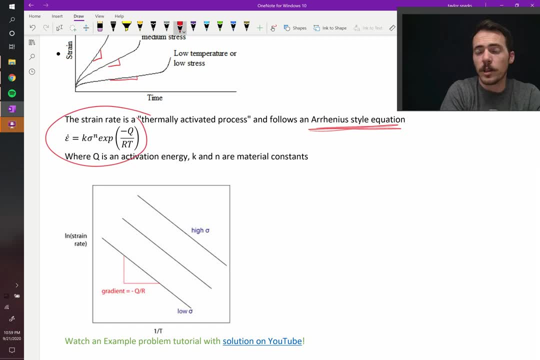 This is not a linear equation right here, but we can make it look linear by doing the following: We need to take the natural log of the strain rate. take the natural log of the strain rate. then we have to take the natural log of both. 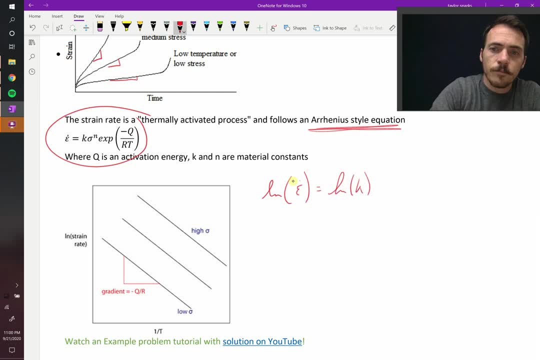 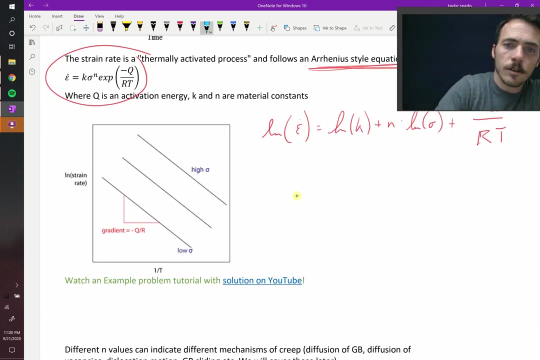 sides, it's going to equal natural log of k plus n times the natural log of stress, plus negative q over RT. okay, So we can make this look linear. now, If you plot this this right, here could be y Plotting this against 1 over T. 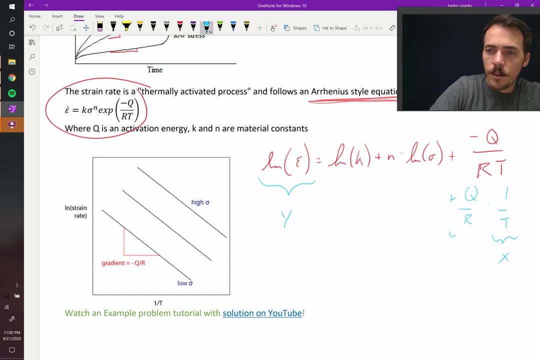 this becomes x, this becomes m and these two become b. So y equals b plus mx. So we were able to linearize it or, in other words, as you can see, as it's written here, the slope of this, if you plot the natural log of the 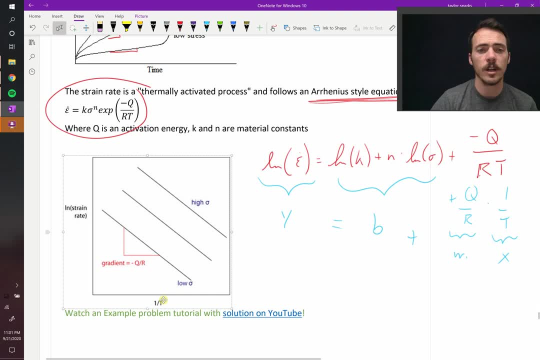 strain rate against 1 over temperature, 1 over temperature in kelvin. you should be able to have that and set it equal to negative q over R. and since R is a constant, the gas constant, 8.314 joules per mole kelvin. all of a sudden you have an activation energy. 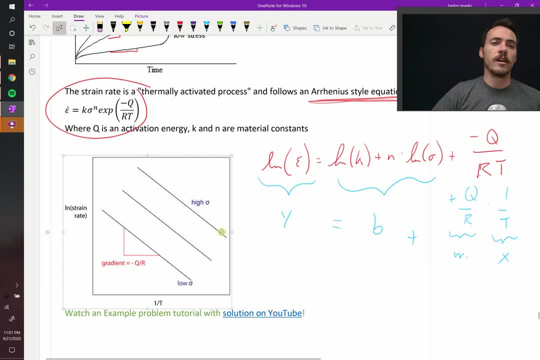 right, So that's pretty fantastic. So this is an example of steady state creep strain rate. Again, you would need multiple equations, since we have three unknowns. we're going to need information to solve three equations and we'll see some examples of that worked. 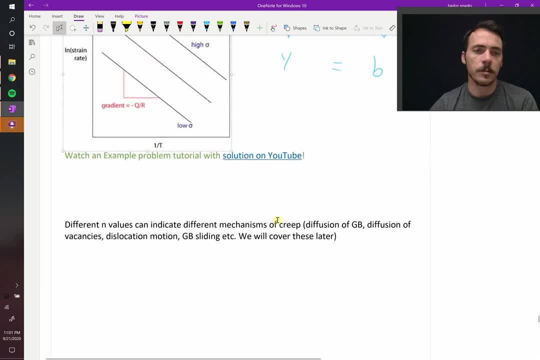 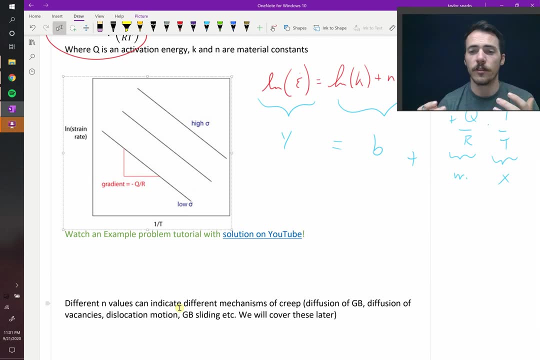 out. Okay. What else can we say about that? Different values of n might indicate different mechanisms of creep. So creep is time-dependent plastic deformation, but that can occur via diffusion along grain boundaries. It could occur through diffusion along what's called vacancies, dislocation, motion grain. 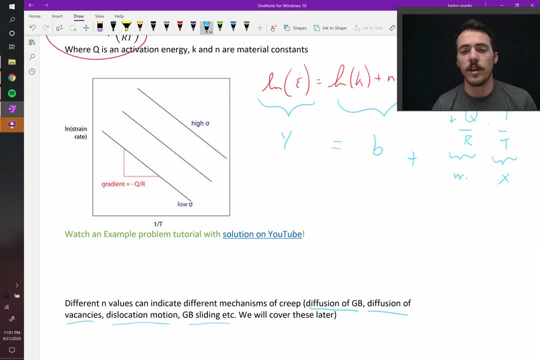 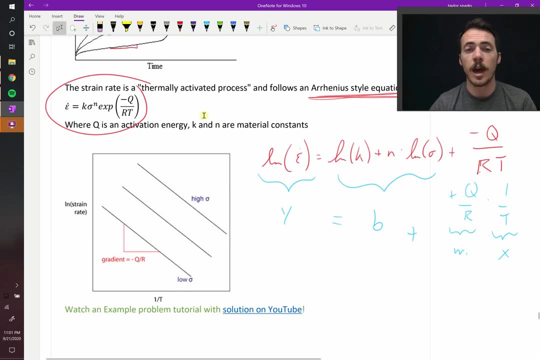 boundary sliding. We haven't talked about those yet in this class. We will get to vacancies and grain boundaries and dislocations in future chapters. But realize that different constants here might happen. in the same material but due to different mechanisms, so different temperature regimes, you might see different constants.